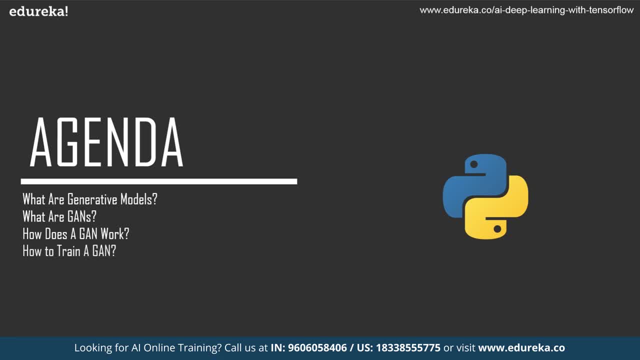 and the need of it, and the advantages as well. moving further, I will tell you a few challenges faced by GANs and finally, to sum up this session, I will discuss a few applications of generative adversarial networks. I hope you guys are clear with the agenda. 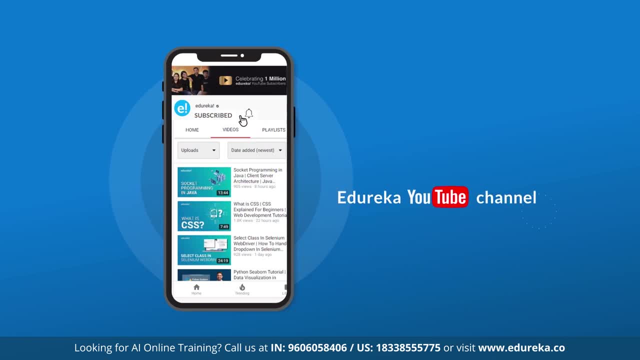 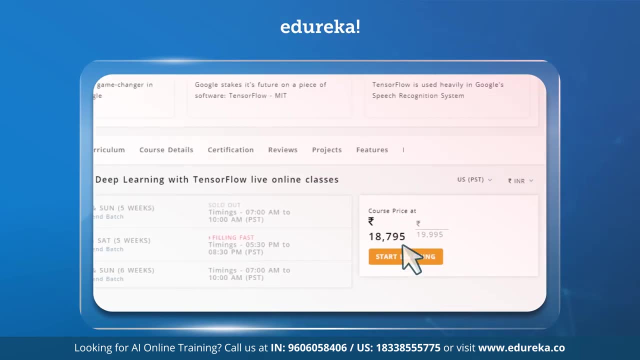 Also, don't forget to subscribe to Edureka for more exciting tutorials, and press the bell icon to get the latest updates on Edureka. Also check out Edureka certification program. The link is given in the description box below. now, without wasting any more time. 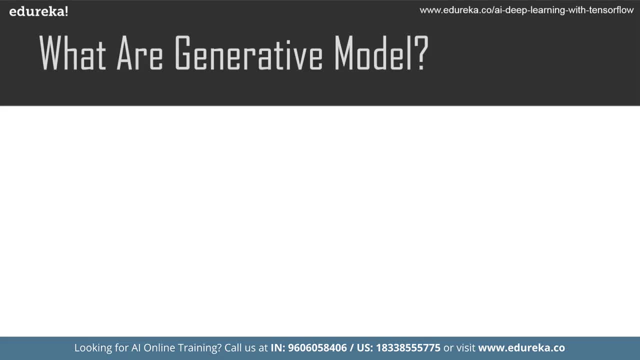 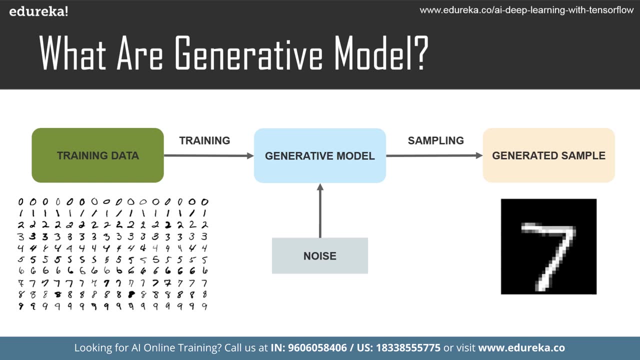 Let us understand what are GANs. So we are going to start with generative models. So generative models are nothing but those models that use an unsupervised learning approach. in a generative model There are samples in the data, that is, input, variables X. 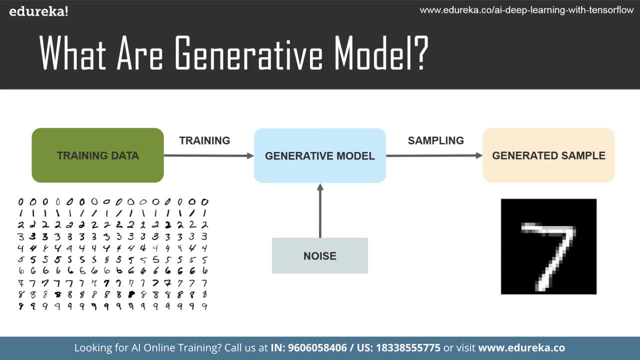 but it lacks the output variable Y and we use the only input variables to train the generative model and it recognizes patterns from the input variables to generate an output that is unknown and based on the training data only in supervised learning We are more aligned towards creating predictive models. 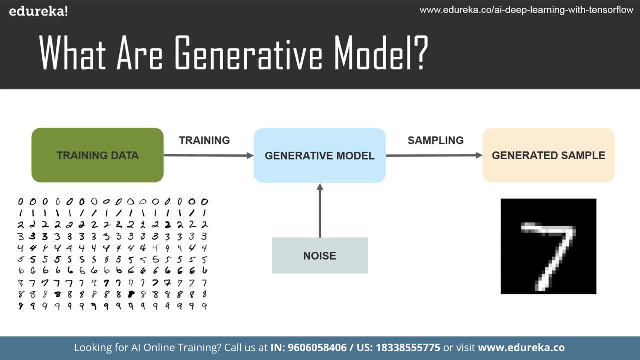 from the input variables, and this type of modeling is also known as discriminative modeling, and in a classification problem, The model has to discriminate as to which class the example belongs to, and, on the other hand, unsupervised models are used to create or generate new examples in the input distribution. 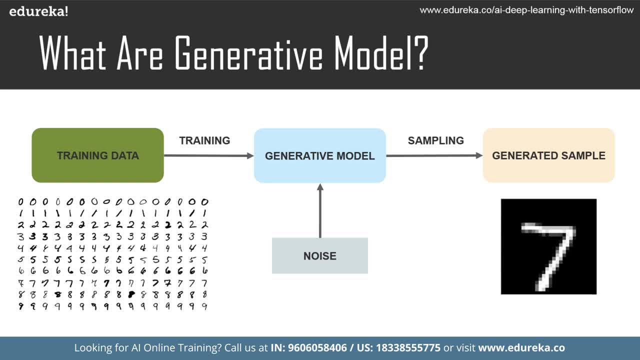 To define a generative model. in layman terms We can say: generative models are able to generate new examples from the sample that are not only similar to the examples but are indistinguishable as well, and the most common example of a generative model is a naive bias classifier. 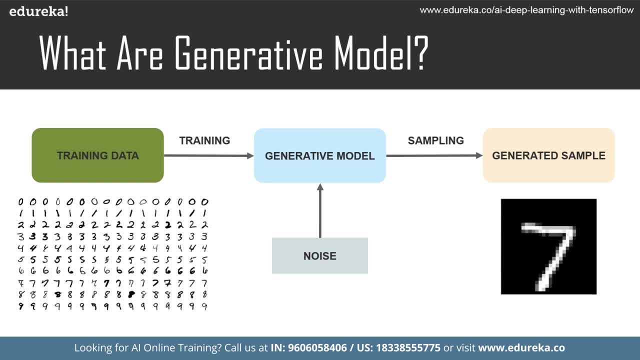 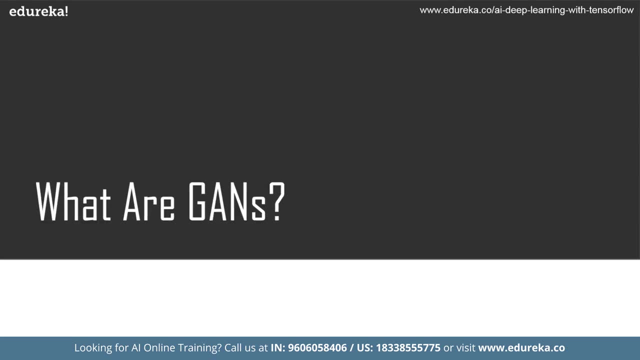 which is more often used as a discriminative model. other examples of generative models include Gaussian mixture model and a rather modern example that is generative adversarial networks. So let us try to understand what exactly are GANs or generative adversarial networks. 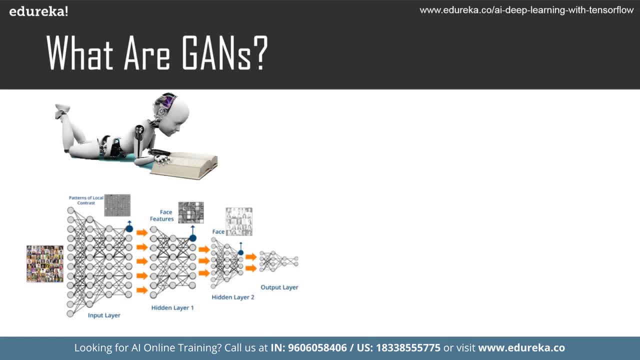 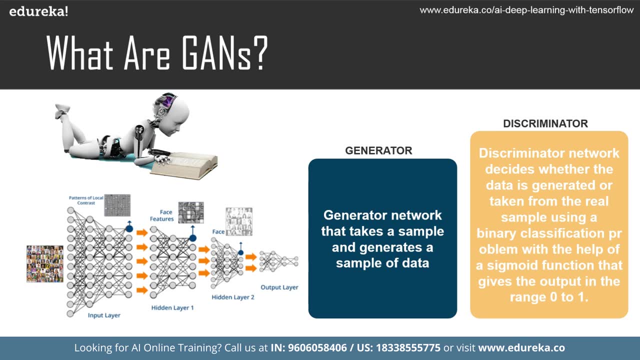 Generative adversarial networks, or GANs, are a deep learning based generative model that is used for unsupervised learning. It is basically a system where two competing neural networks compete with each other to create or generate variations in the data. It was first described in a paper in 2014. 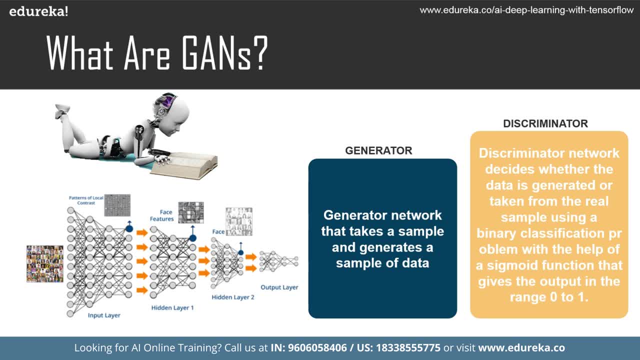 by ENG Goodfellow, and a standardized and much stable model theory was proposed by Alec Radford in 2016,, which is also known as DGC a n also known as DC GAN, or we can call it as deep convalescent and general adversarial networks. 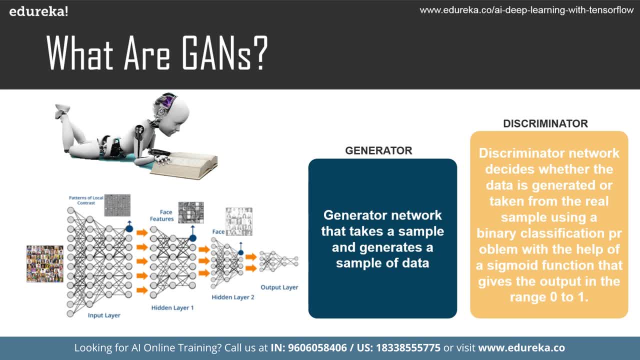 and most of the GANs today use deep convalescent and general adversarial networks. The GANs architecture consists of two sub models known as the generator model and the discriminator model. So a generator network takes a sample and generates sample of data. a discriminator network decides. 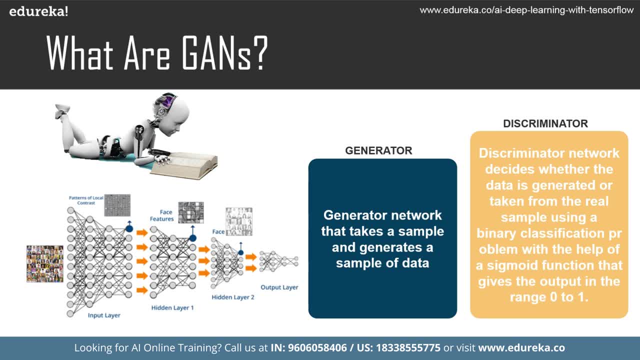 whether the data is generated or taken from the real sample using a binary classification problem with the help of a sigmoid function that gives the output in the form or the range 0 and 1.. So let us go ahead and take a look at how GANs actually work. 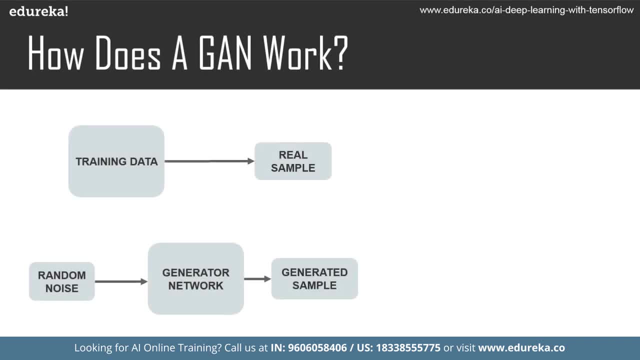 To understand how GANs work. Let's break it down So: generative means that the model follows the unsupervised learning approach and is a generative model. when we talk about adversarial, The model is trained in an adversarial setting and Network simply means for the training of the model. 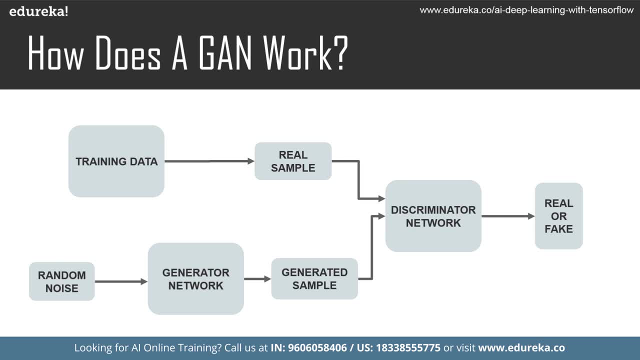 We use the neural networks as artificial intelligence algorithms. in GANs, There is a generator network that takes a sample and generates a sample of data, and after this the discriminator Network decides whether the data is generated or taken from the real sample using a binary classification. 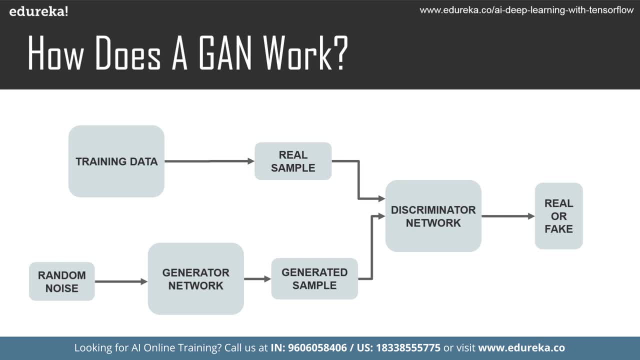 problem with the help of a sigmoid function that gives the output in the range 0 to 1. the generate a model analyzes the distribution of the data in such a way that, after the training phase, the probability of the discriminator making a mistake maximizes and the discriminator, on the other hand, is based on a model. 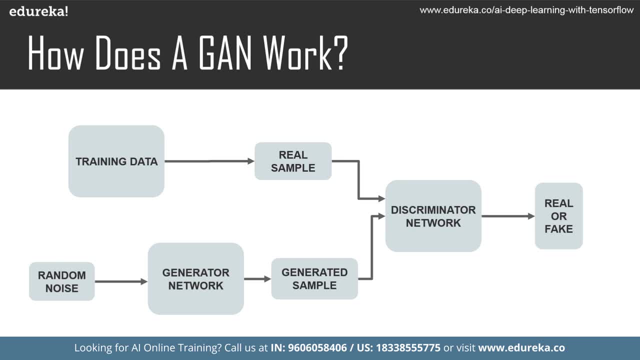 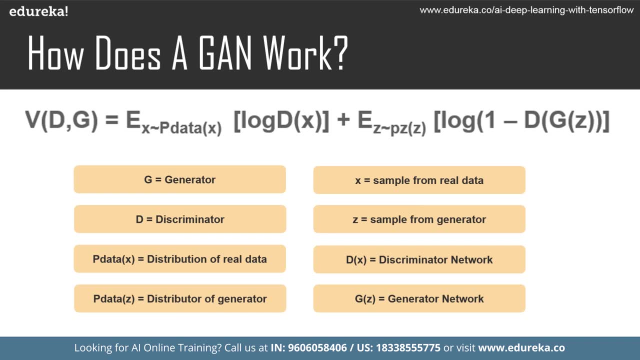 that will estimate the probability that the sample is coming from the real data or not, the generator. the whole process can be formalized in a mathematical formula. So G over here is the number which is generator. D is equal to discriminator P data. X is the distribution of real data. P data. Z is the distributor. 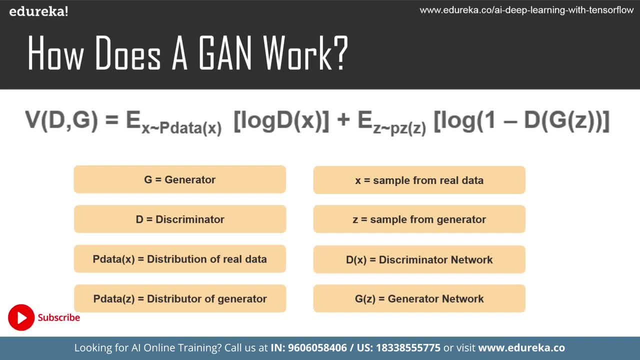 of generator. X is the sample from the real data and Z is the sample from generator, where DX is the discriminator Network and GZ is a generator Network. So let's take a look at the flow chart once again, guys. So we have the training data. 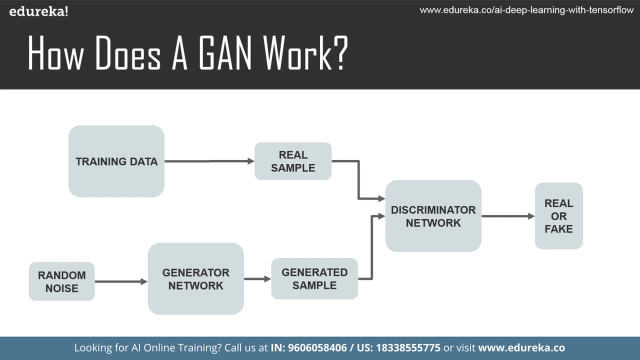 which is going to give the real sample, and the generator Network is going to generate the sample from the random noise or the examples and then it will go to the discriminator Network where it's going to check if the sample that is coming is real or fake. 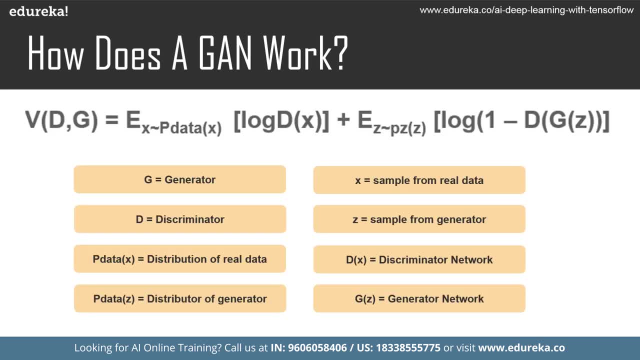 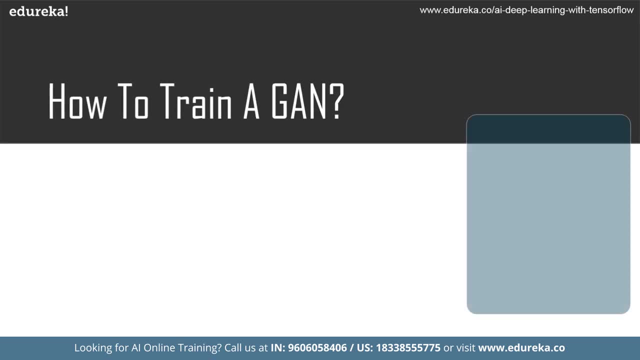 So that is how again actually work. Now let's take a look at the training phase, like how a generative adversarial Network is actually trained. So it happens in two phases, guys. So the first phase is where we train the discriminator and we actually freeze the generator. 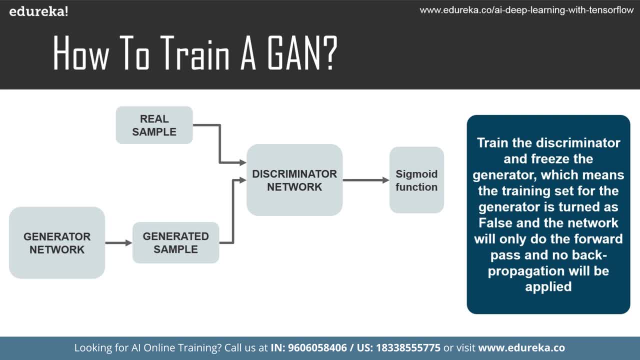 which means that the training set for the generator is turns back to false and the network will only do the forward pass and they will not be any back propagation. Basically, the discriminator is trained with real data and checks if it can predict them correctly, and the same with the fake data to identify them as fake. 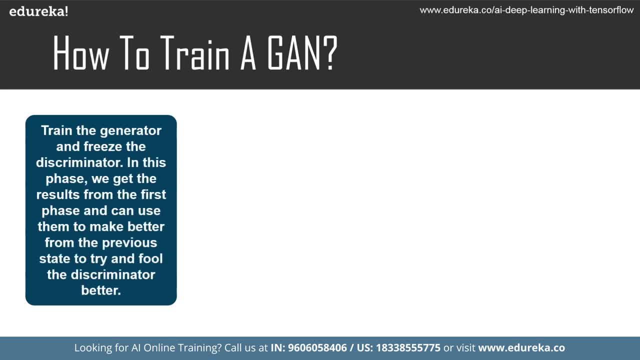 After this there's the second part, where we train the generator and freeze the discriminator. So we get the result from the first phase and we use them to make better from the previous state, to try and fool the discriminator better. So to understand this in the layman's term: 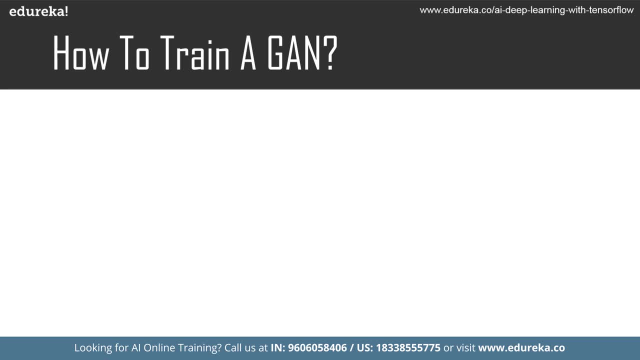 I'm going to tell you a few steps for training, like how you should start. So the first step is you have to define the problem. You have got to define the problem and collect the data. After this, the second step is you have to choose the architecture of gang. 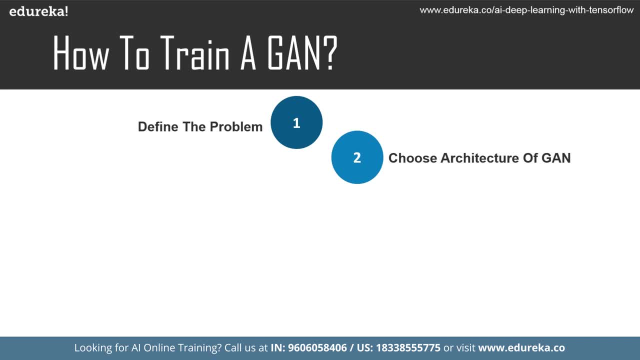 So in this step, depending on your problem, you have to choose how your gang should look like. The third step is training the discriminator on real data. So we train the discriminator with real data to predict them as real For n number of times, or we call it epochs as well. 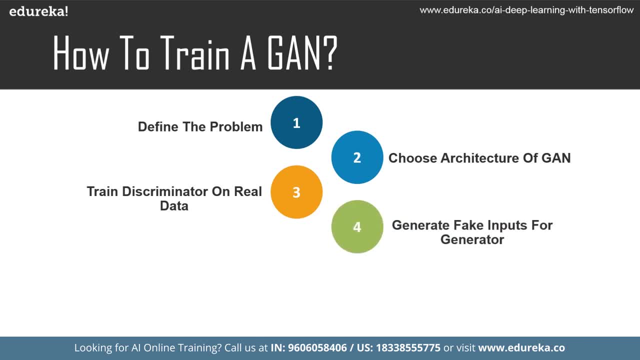 and then we generate the fake inputs from the generator. So in this step, we are going to generate the fake samples from the generator and the next step is we train the discriminator on fake data. So, whatever samples are generated from the generator Network, you're going to train the discriminator. 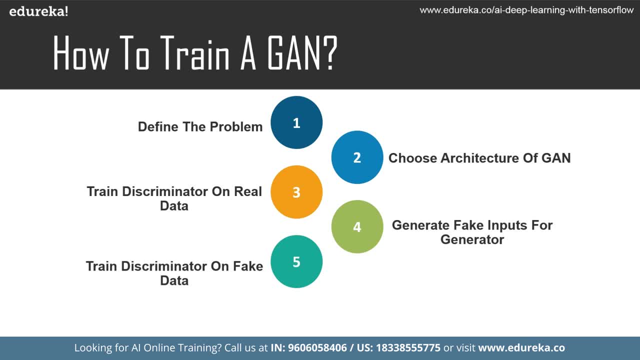 to predict the generator data as fake. So that's how we know that discriminator is actually predicting the values as correctly. and the last step is we train the generated with the output of discriminator. So, after getting the discriminator predictions, we train the generator to fool the discriminator. 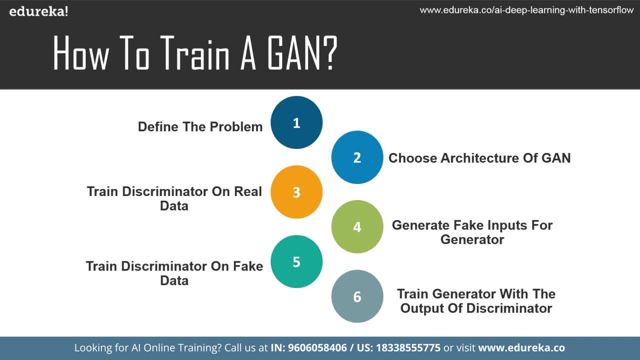 So that's how we train the Gantt to actually get our solution from the problem, which is like defining the problem. So you'll understand this when I'm talking about the applications, guys. no worry, Now let's go ahead and take a look. 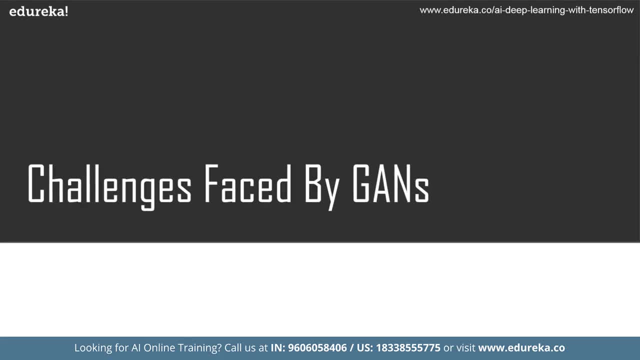 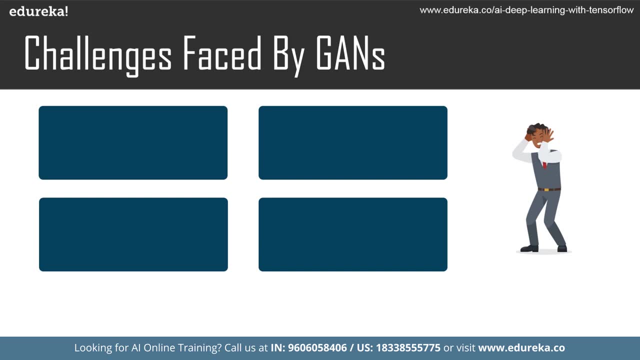 at a few challenges of generative adversarial networks. So the concept of Gantt's is rather fascinating but there are a lot of setbacks That can cause a lot of hindrance in its path. Some of the major challenges faced by Gantt's are the first: 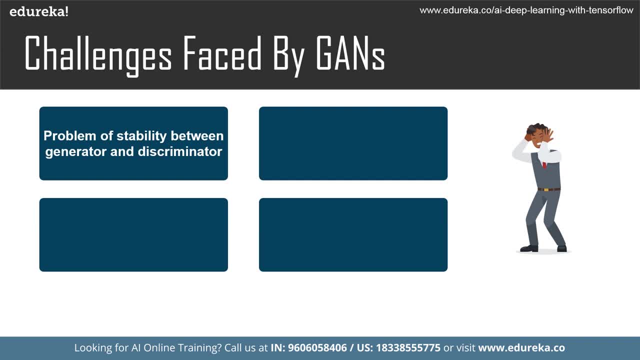 one is the stability. So there has to be a stability, that is required- between discriminator and the generator Network, Otherwise the whole network would just fall. for example, in case, let's say, if the discriminator is too powerful, the generator will fail to train altogether, won't be able. 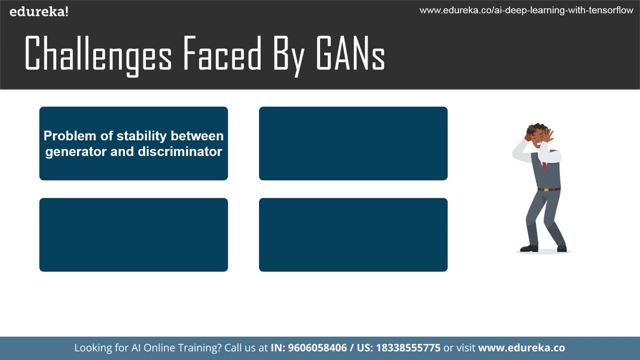 to push fake samples to the discriminator and it will always identify them as fake. and let's say, if the network is too lenient, the discriminator Network is too lenient, So any image that would be generated by the generator Network would make the network useless. 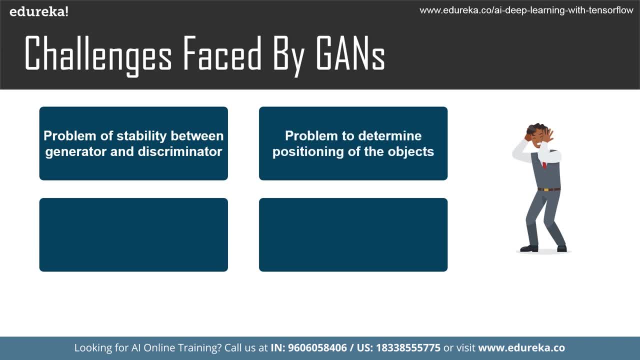 The next challenge that is faced by Gantt's is Gantt's fail miserably in determining the positioning of the objects in terms of how many times the object should occur at that location. Suppose we have a image in which we have, let's say, three dogs. 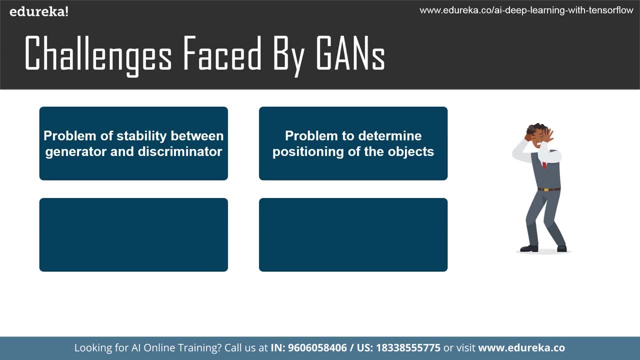 with two eyes and sometimes again will fail to, you know, determine the positioning of the objects in terms of it will generate an image with like one dog and six eyes. So that's kind of a problem that we face while working on Gantt's and the next challenges. 3D perspective troubles Gantt's. 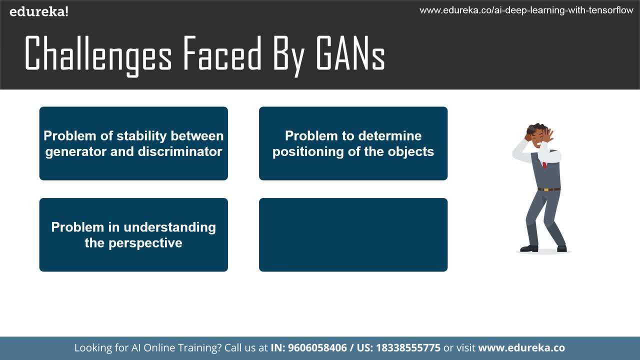 as it is not able to understand the perspective also, So it will often give a flat image for a 3D object. So that's one challenge that we face with Gantt's as well, and Gantt's have a problem of understanding the global objects. 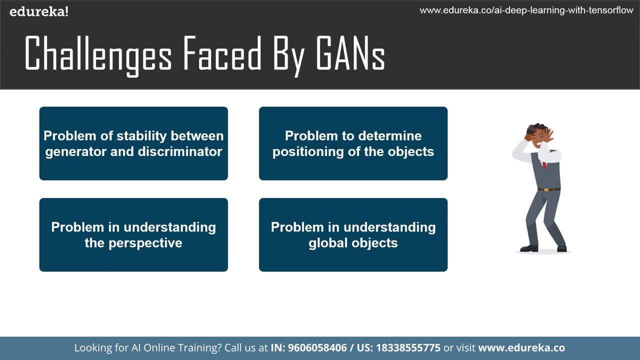 and it cannot differentiate or understand a holistic structure. If you're talking about trees or if you're talking about flowers, that's a problem that Gantt's will follow and, last but not least, newer types of Gantt's are more advanced that I've talked about. that is deep convolutional. 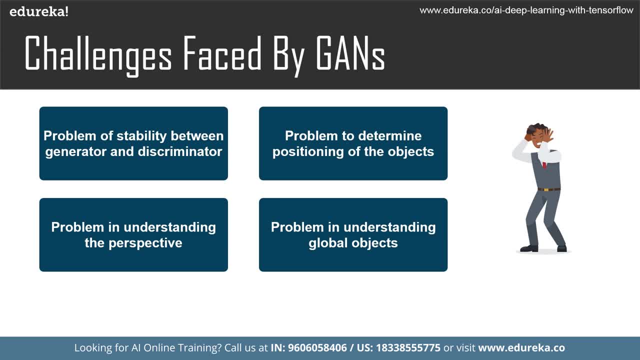 generative adversal networks and are expected to overcome these shortcomings altogether, So we don't have to worry about these. These are the shortcomings that we face with normal Gantt's, the initial generative adversal networks. now that they have become more advanced. 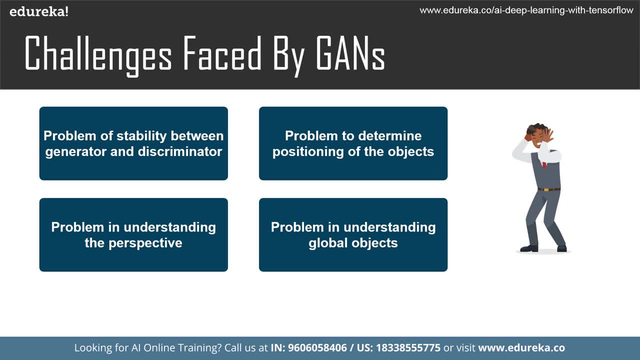 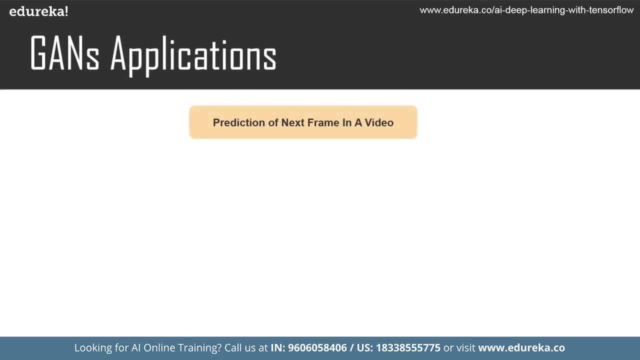 They actually overcome these shortcomings. So you don't have to worry guys. So, last but not the least, I want to talk about a few applications of generative adversal networks. So the first one is prediction of next frame in a video. So let's say, the prediction of future events in a video frame. 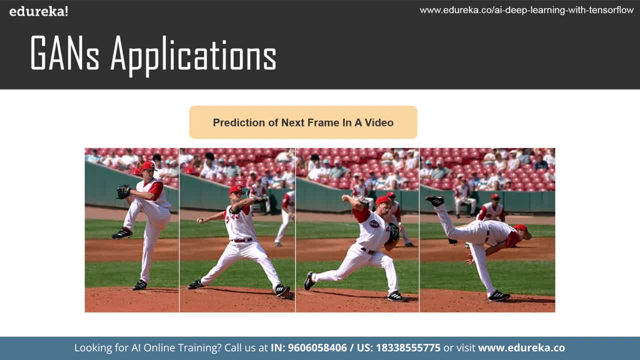 is made possible with the help of Gantt's and DVD. Gantt, or we can call it as dual video discriminator. Gantt can generate a 256 by 256 videos of notable Fidelity, up to 48 frames in length, and this can be used for various purposes. 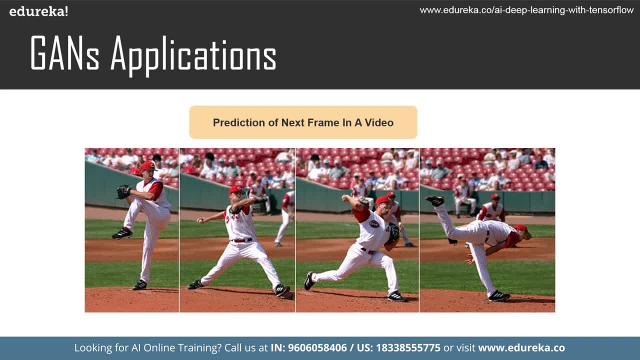 including surveillance, in which we can determine the activities in a frame that gets distorted due to other factors like rain, dust, smoke, Etc. So the possibilities are immense with this. If you are able to predict the next frame in a video, that actually helps in a lot of things. 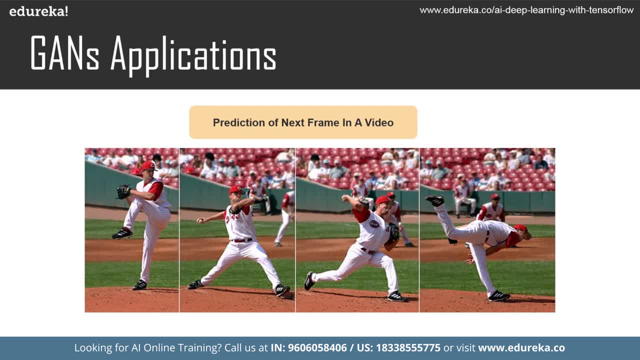 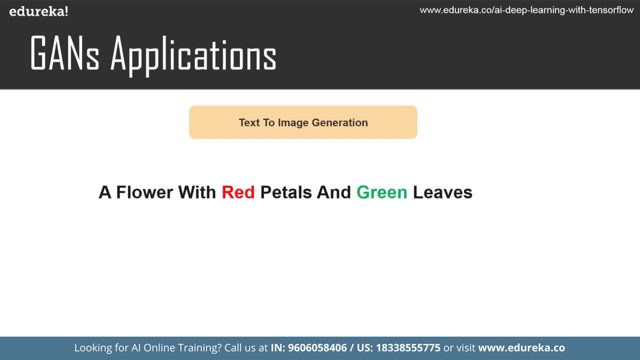 like surveillance, security, and we can predict outcomes based on these frames that we generate from a video. after this comes the text to image generation, So basically object-driven. attentive Gantt, which is also known as object Gantt, performs the text to image synthesis in two steps. 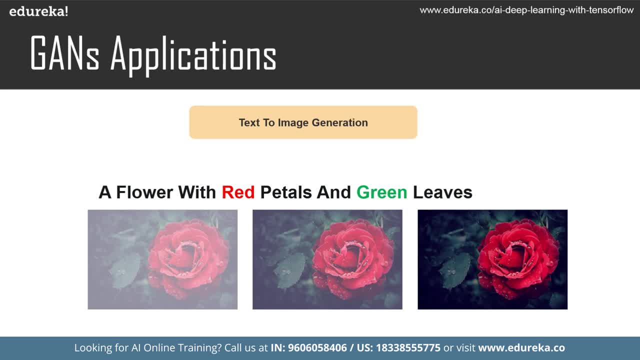 So the first step is generating the semantic layout and then generating the image by synthesizing the image by using a deconvolution. al image generator is the final step. So this could be used intensively to generate images by understanding the captions, the layouts and refined details by synthesizing the words. 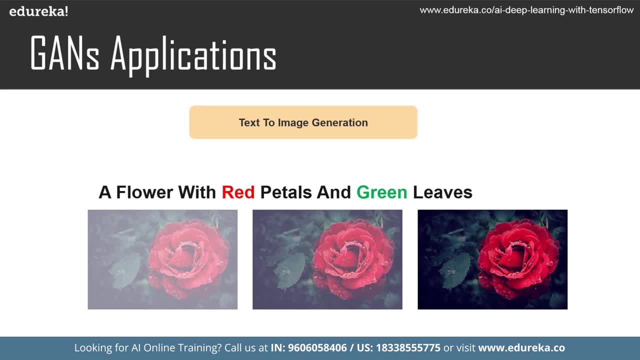 and there is another study about the story Gantt's that can synthesize the whole storyboard from mere paragraphs. So that's actually very good idea If you're talking about gas, so you can just give a few layouts and captions based on that. 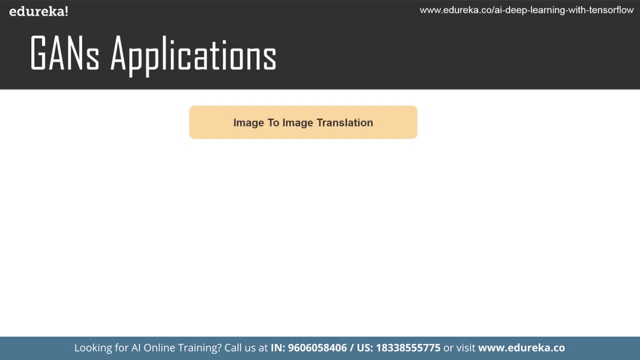 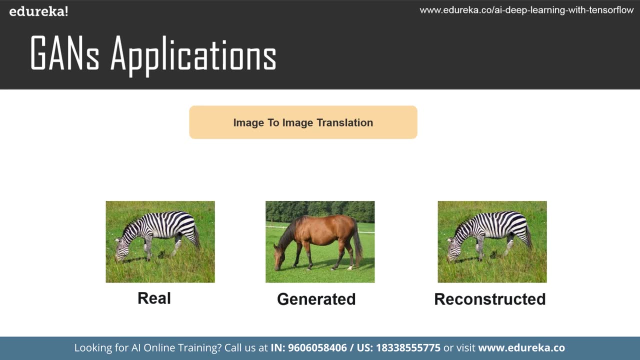 It will generate image for us. talking about the next application, We have image to image translation. So pics to pics is a model which is designed for general purpose: image to image translation. So let's say we have three images, We have a real image, then we'll be having a generated image. 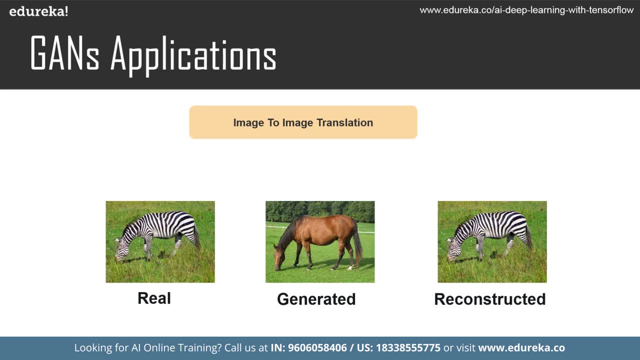 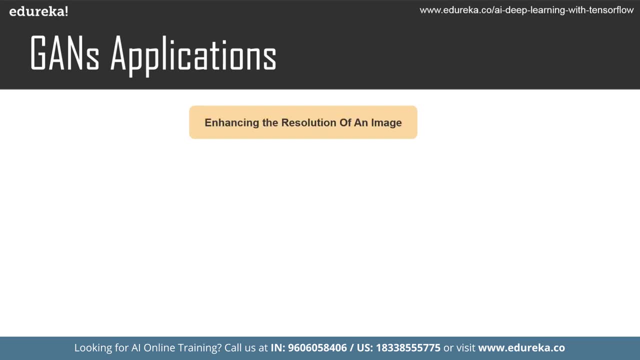 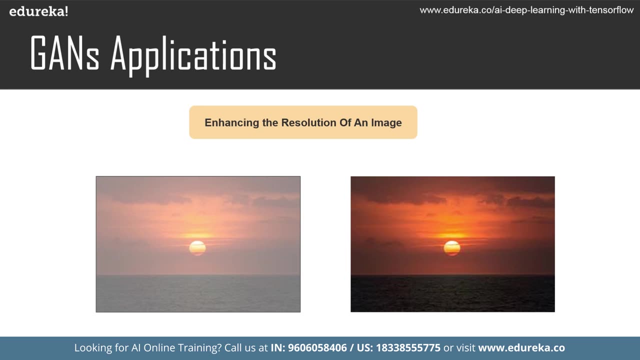 which is basically a fake, and then it will be reconstructed the previous image which was real. So this is our major image translation work, guys. and after this we have enhancing the resolution of an image. So super resolution generative adversarial Network, or also known as SR, Gann is a Gann. 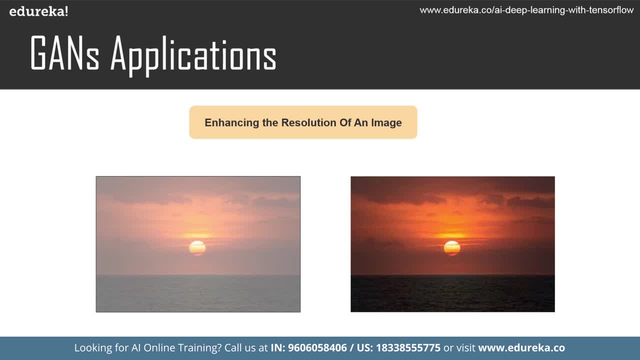 which can generate the super resolution images from low resolution images with finer details and better quality. So this is actually a very good application of Gans guys. The applications can be immense. So you imagine a high resolution, higher quality image with finer details generated from a low resolution image, the amount of help. 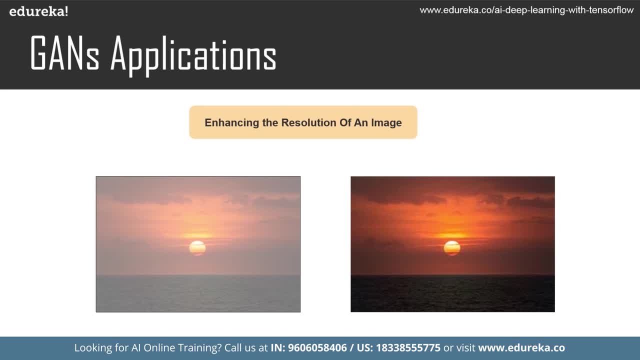 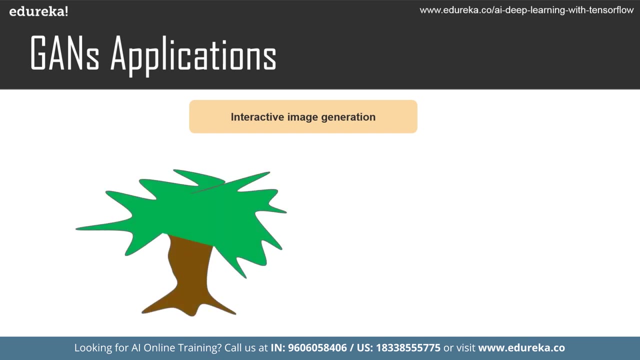 it would produce to identify details in lower resolution. images can be used for wider purposes, including surveillance. We can use it for documentation security. We can use it for detecting patterns, Etc. And last but not least, we have interactive image generation. So Gans can be used to generate interactive images as well. 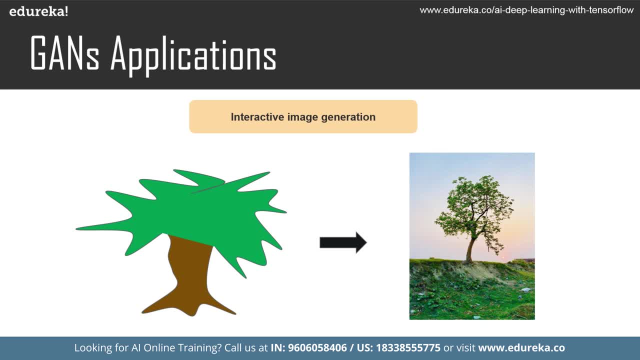 and computer science and artificial intelligence library, also known as CSA, IL, has developed a Gann that can generate 3D models with realistic lighting and reflections enabled by the shape and texture editing, and, more recently, researchers have come up with a model that can synthesize a reenacted face animated. 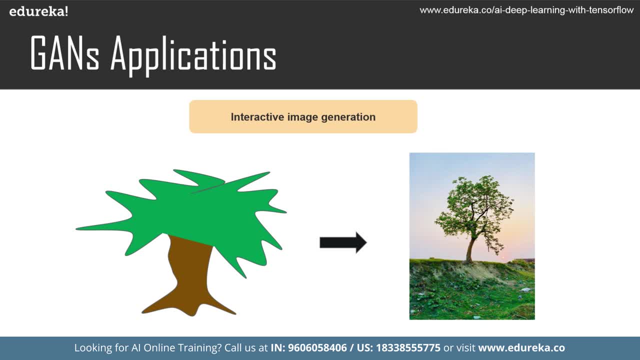 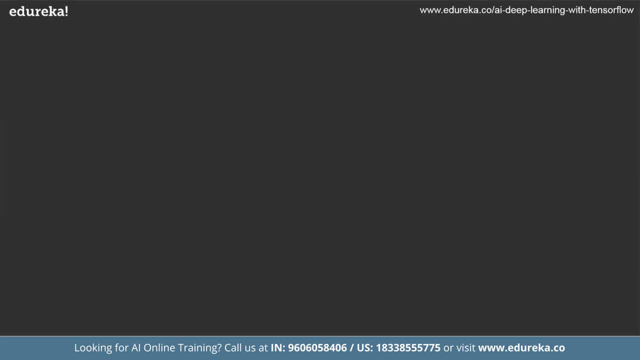 by a person's movement while preserving the appearance of the face at the same time. There are a lot more applications we can work on. So this brings us to the end of this session, guys, where we have learned what our Gans, how it works and what are the challenges faced. 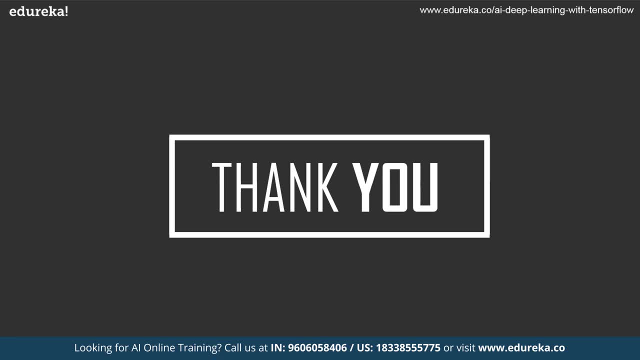 by Gans, including the applications of generative adversarial networks. So in the end of the session I just want to tell you guys, don't forget to subscribe to edureka for more exciting tutorials and press the bell icon to get the latest updates on edureka. 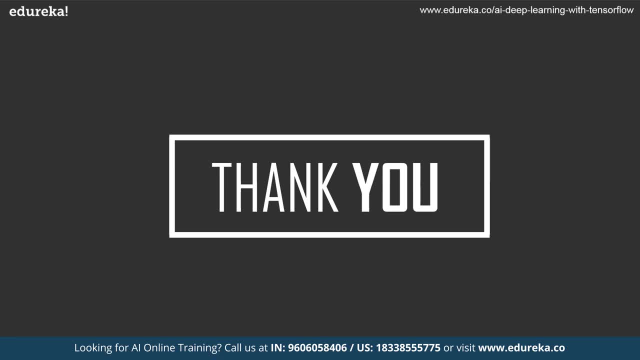 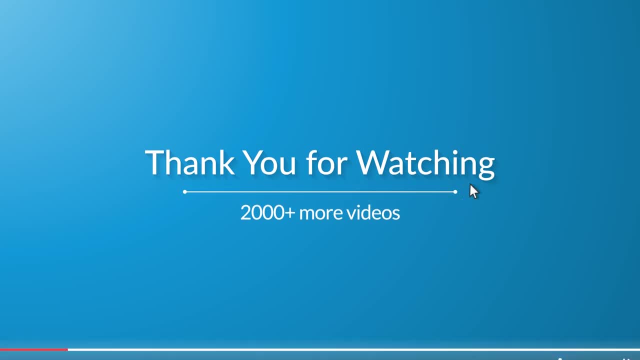 Also check out edureka certification program. The link is given in the description box below. Happy learning, Thank you. I hope you have enjoyed listening to this video. Please be kind enough to like it and you can comment any of your doubts and queries.